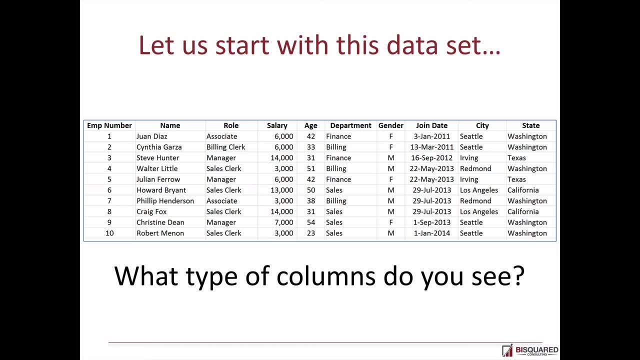 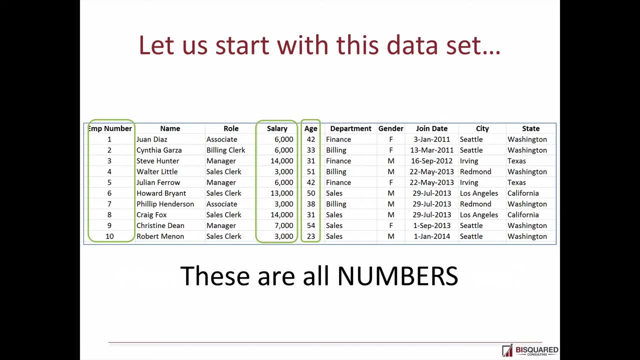 non-numbers, but predominantly it would be text. So let's look at this sample data set. So what type of columns do you see? So these are all the numbers. I see employee number, I see salary, I see age. These are all the numbers, And measures are nothing but numbers. 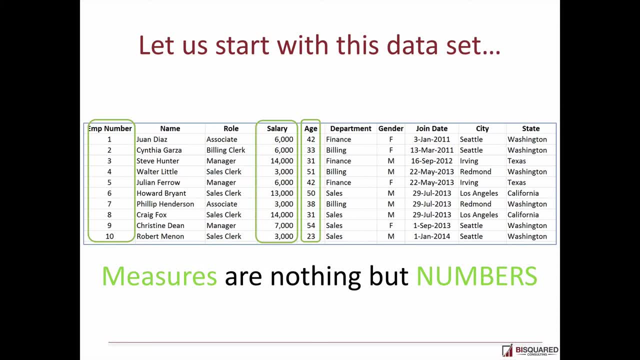 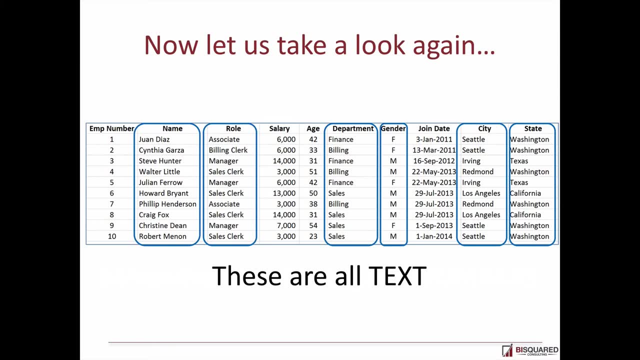 That's all. Whenever you hear the word measure, just think of numbers. That's all. Whenever you hear the word measure, just think of numbers. That's all. That's all measures are. And let's take a look at the data set again Now. I have highlighted the 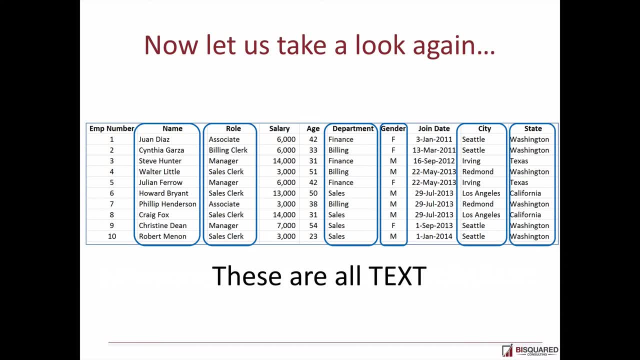 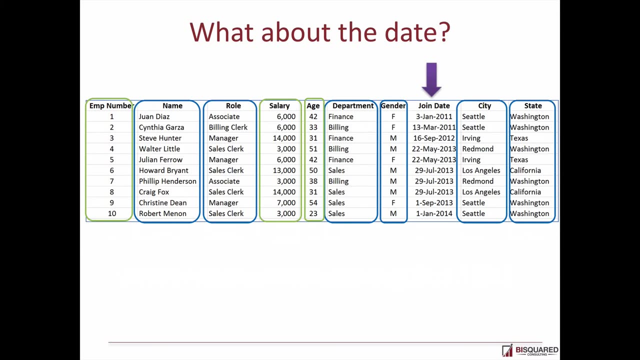 text. These are all the text. There's name, role, department, gender, city, state. They are all text, and dimensions are nothing but text. So that's all. And if you look closely, what about the date? I have not highlighted that Date is neither green nor blue. So what about the date? So the date is. 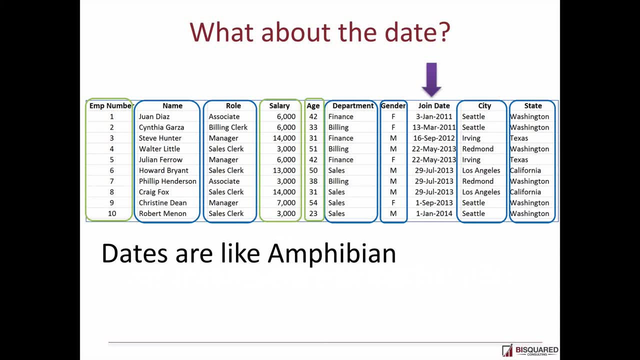 like an amphibian, right. So we know things like frogs. they can live on water, they can live on land. In the same way, dates can behave like dimensions, like text- And most of the times they do, But there are some times they can behave like numbers. They do have properties like number, like. 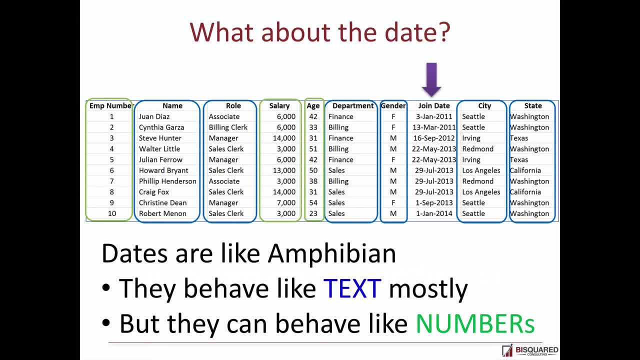 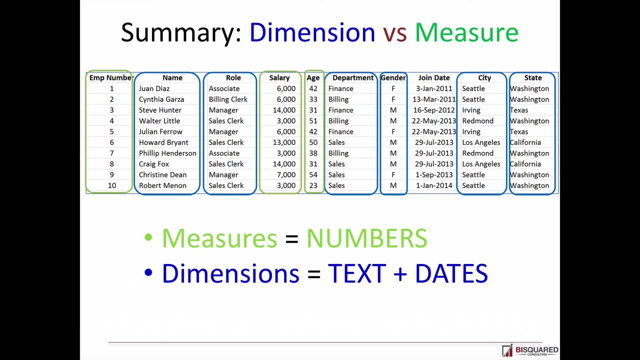 min and max and stuff which we'll cover later in detail, Right? So dates fall in between. So let's summarize this. So dimensions are numbers. So let's summarize this. So dimensions are numbers Are nothing but text, And you add dates to that, because that that dates are also behaving like